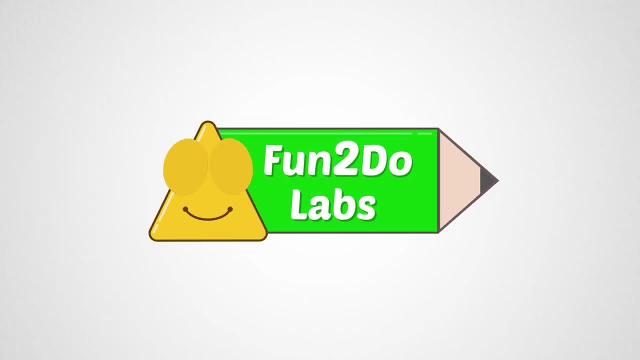 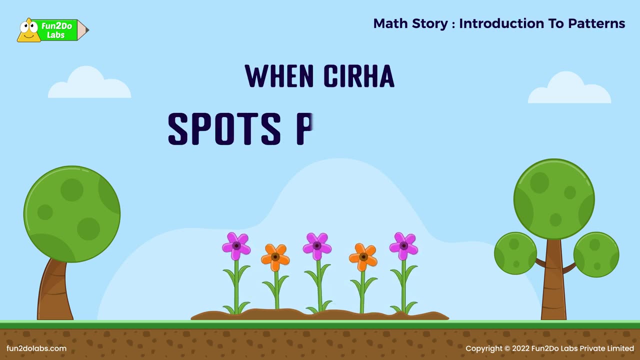 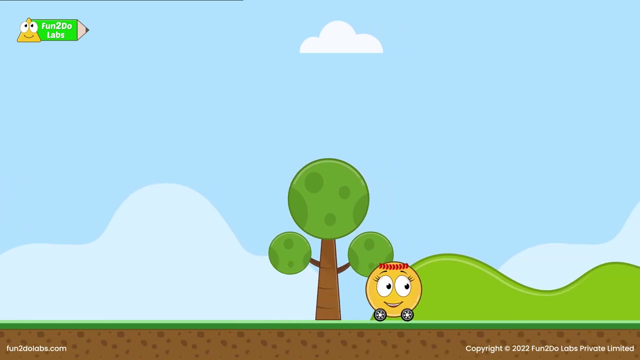 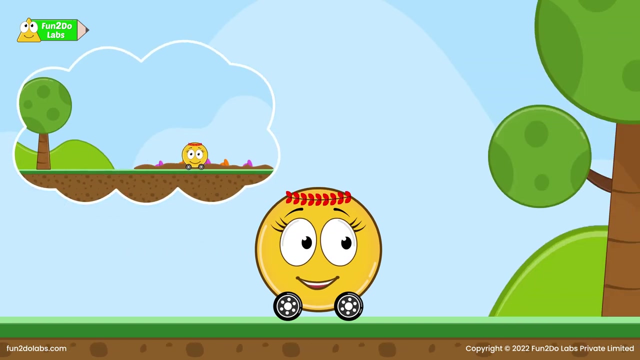 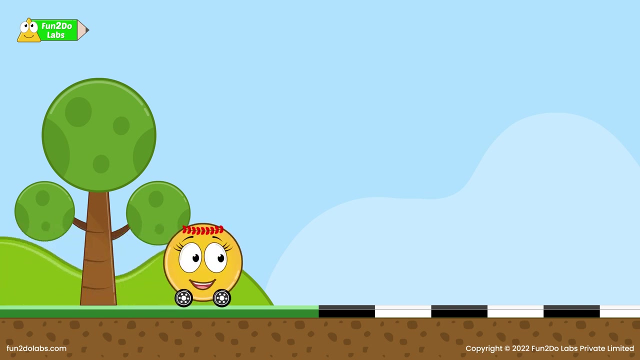 Matt's Story. Introduction to Patterns. When Sirha spots patterns, Sirha is happily walking. Uncle Matt is organising a gardening competition. Wow, That would be fun. Gardening is Sirha's favourite hobby too. On the way she sees that the black and white stripes on the road are repeating. 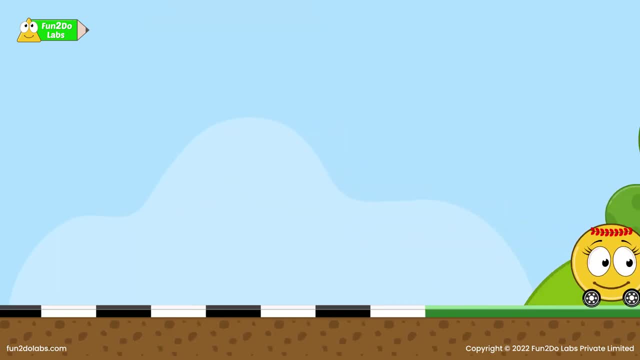 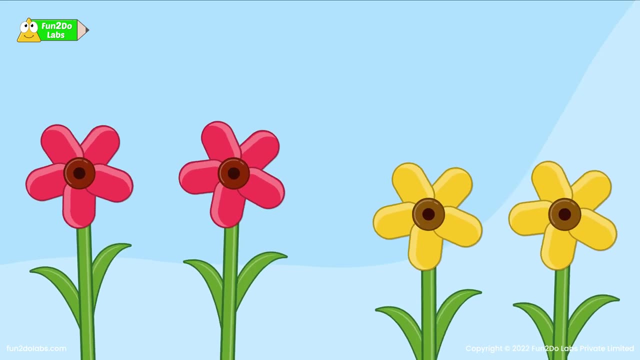 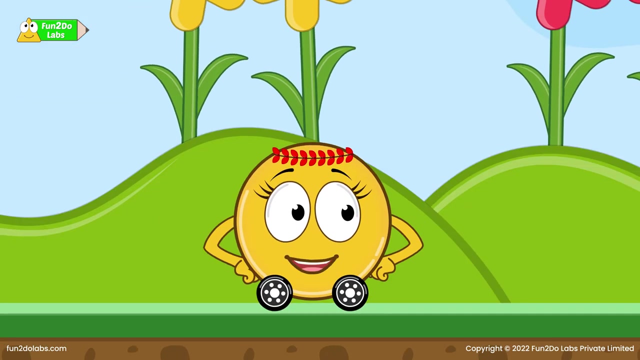 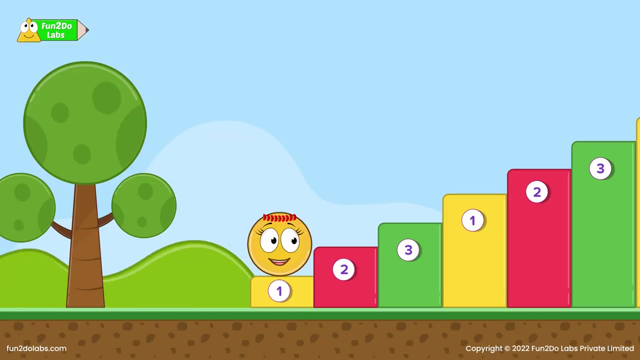 Black, white, black, white, Red flowers, yellow flowers, Red flowers, yellow flowers, Red flowers, yellow flowers, They seem to repeat as well. Strange, Moving ahead, Sirha sees some steps: One, two, three. One, two, three. 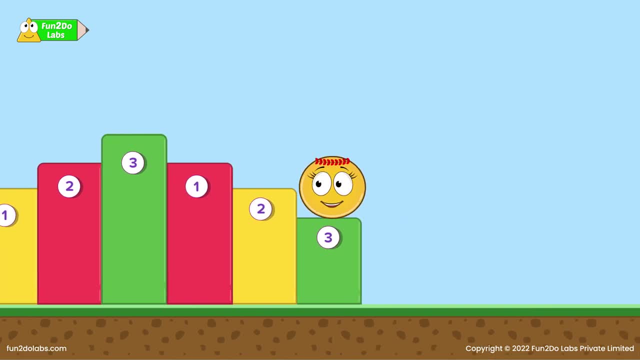 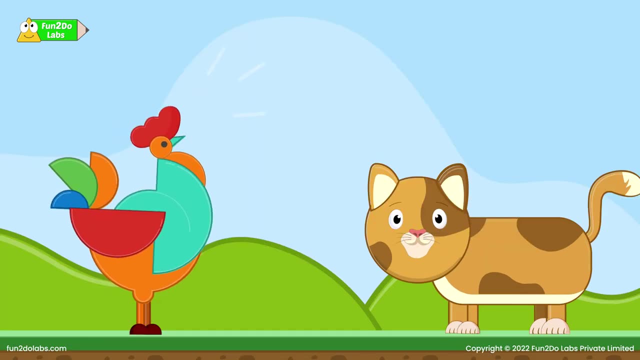 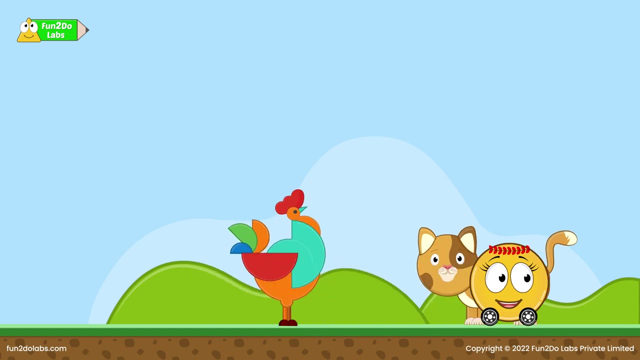 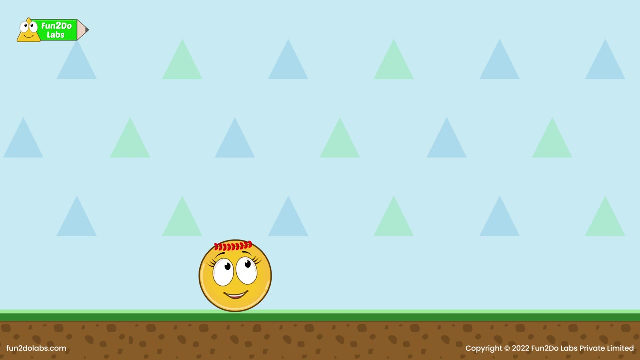 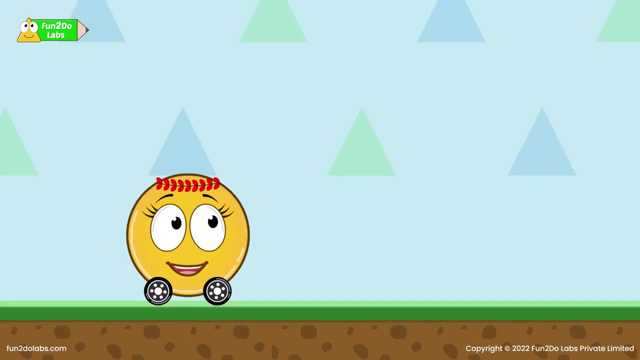 One, two, three- The numbers are also repeating here. A cat and a hen cry. She is surprised and quickly rushes to Uncle Matt's place. As she moves ahead, Sirha spots a huge wall: Blue triangle, green triangle. blue triangle, green triangle. 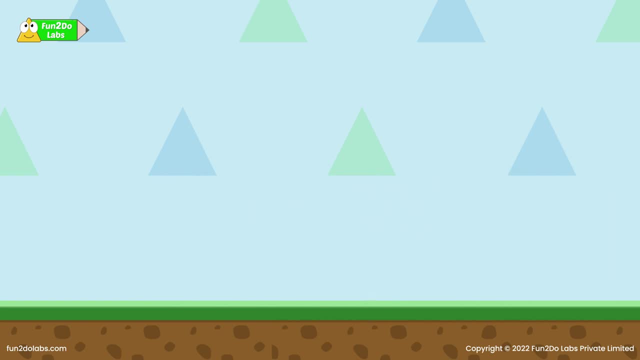 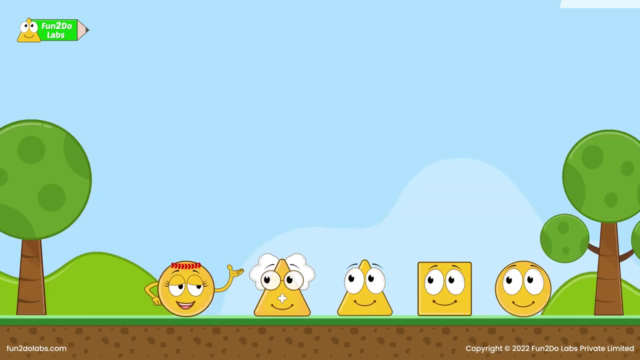 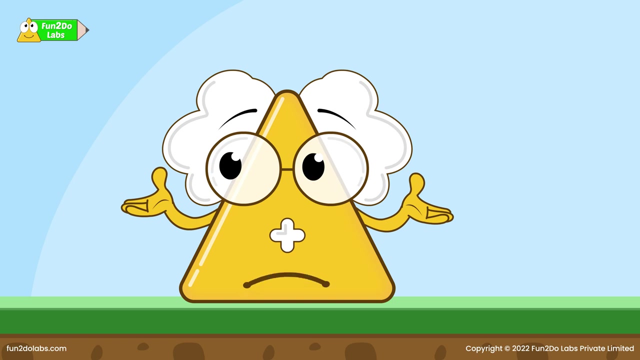 The triangles are repeating on the wall. Uncle Matt, come here fast. Sampertown has been acting strange today. Everything is repeating, Repeating What is repeating. Sirha narrates, Sirha narrates, Sirha narrates. Now she first spotted repeating black and white lines. 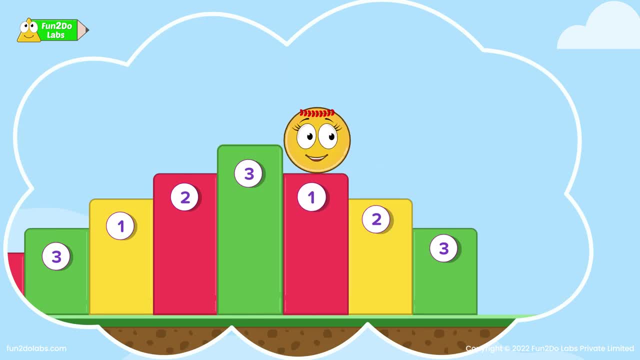 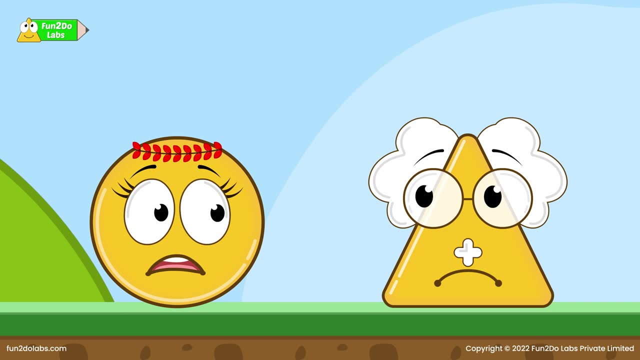 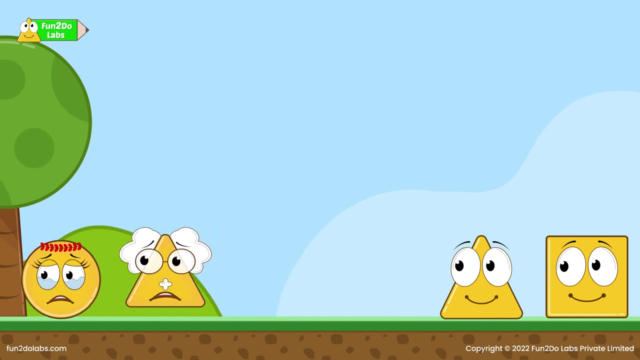 Then repeating flowers, Then numbers, then animal sounds, Then numbers, then animal sounds, then depende the repeating triangles. Hearing this Uncle Matt bursts into laughter. Hearing this Uncle Matt bursts into laughter. This disappoints Sirha and she starts sobbing. 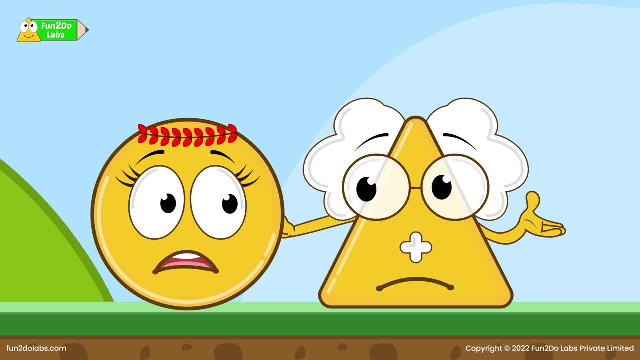 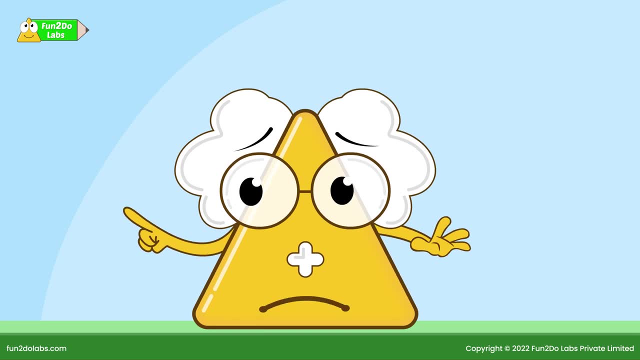 Uncle Matt apologises for laughing at her and decides to calm her down. Sirha, all these lines. Sirha, all these lines flowers. Sirha, all these lines Shapes, numbers that were repeating were actually making a pattern. Sira is still clueless. 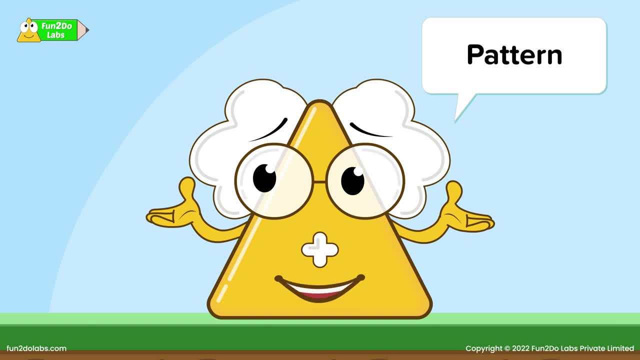 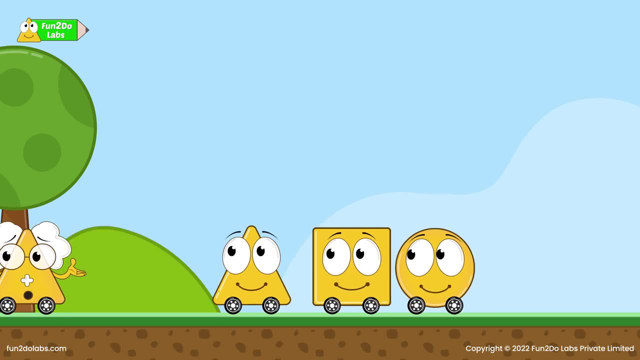 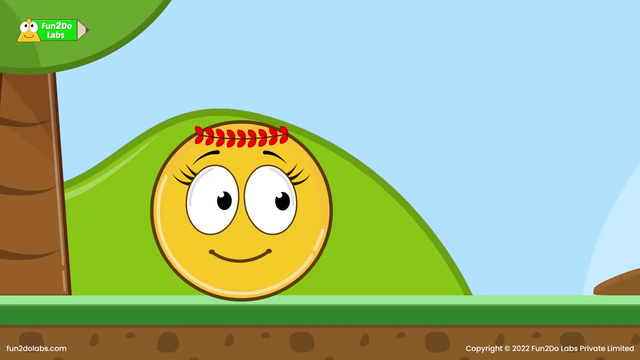 Anything that repeats itself following a rule is forming a pattern. Patterns are all around us. Finally, Sira is happy. Let's start the competition. All four of them take their places and start gardening. Sira decides to make a flower garden using a pattern. 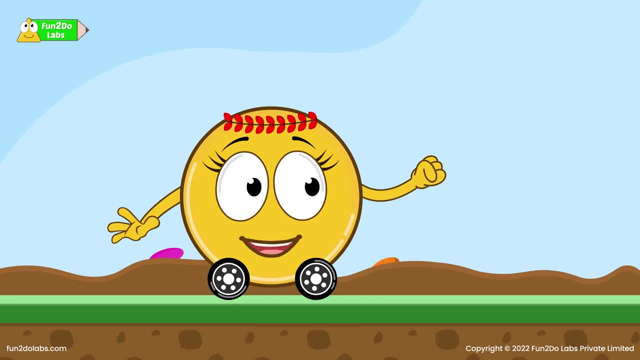 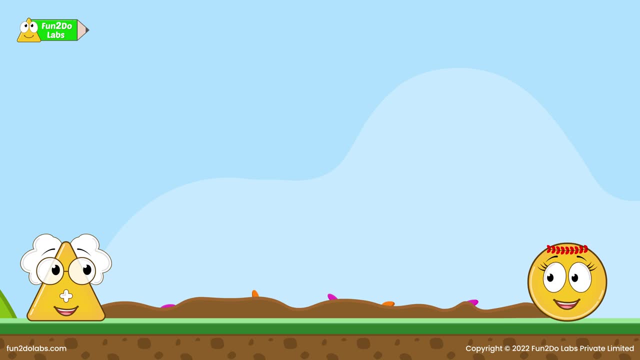 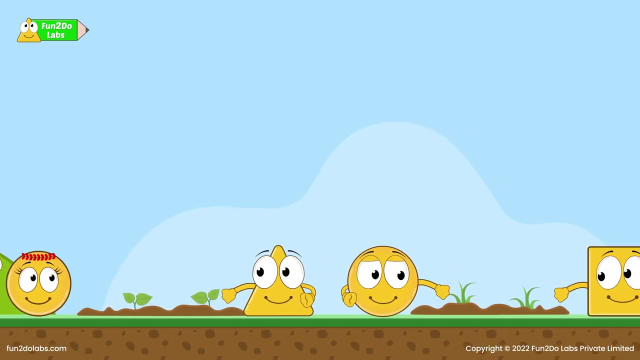 Pink flower seed. orange flower seed. pink flower seed. orange flower seed. pink flower seed. She says and places her beautiful plant seeds following a pattern: Treeho is growing vegetables and Sirho and Squirro are growing small plants. The winner will be announced after a month. 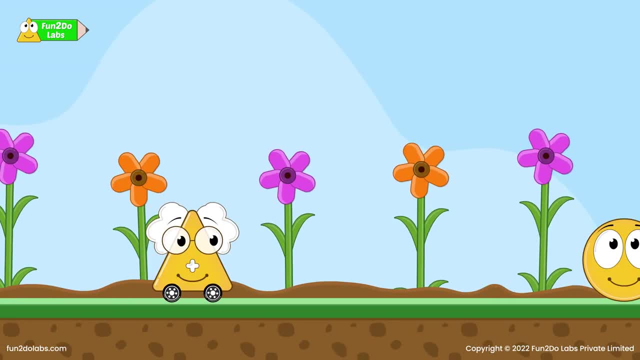 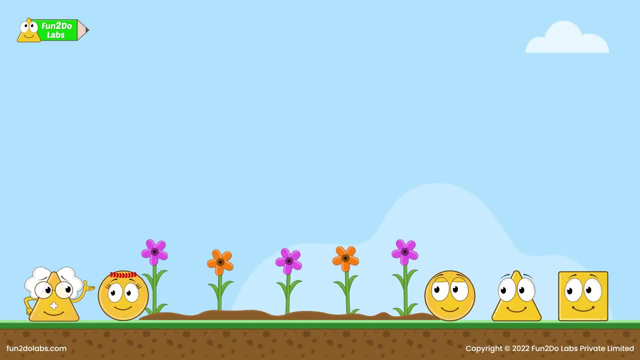 It is time to announce the results. Uncle Math closely observes All of your gardens look good, But Sirha's garden looks amazing. Look at the colorful flowers arranged in a pattern. Clearly, Sirha is the winner. Hip, hip, hooray. Sirha is the winner. 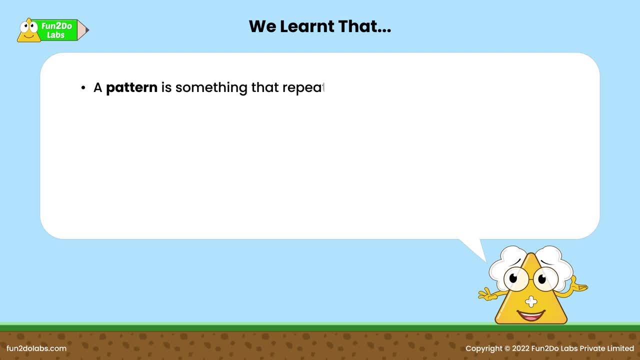 We learned that a pattern is something that repeats itself following a rule. Patterns can be formed using shapes, numbers, colors and many other things. Patterns are all around us. We should never laugh at others. Instead, we should hear them out and make them feel better. 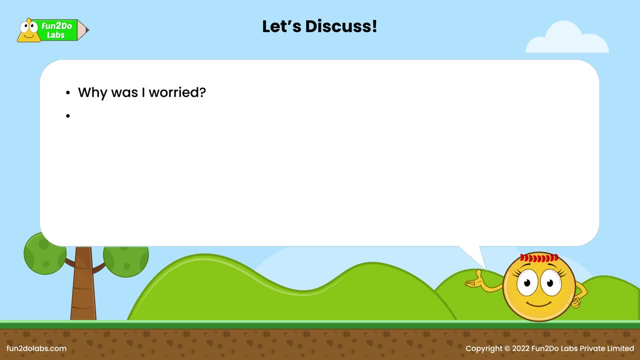 Let's discuss. Why was I worried? What are patterns? Explain How I found various patterns around Sampatown. Can you spot some patterns around you as well? I became sad when everybody laughed at me. How would you feel if you were in my place? 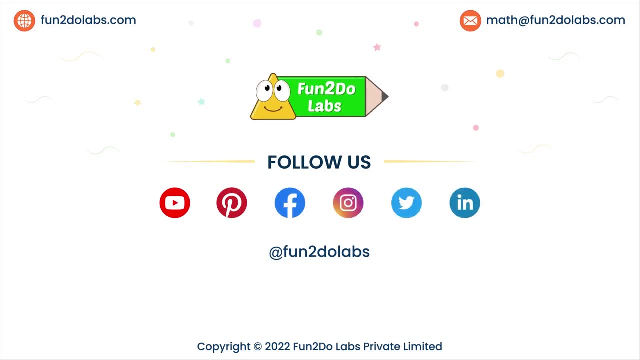 Follow us on Fun To Do Labs, to enjoy watching more such math stories, songs and games.